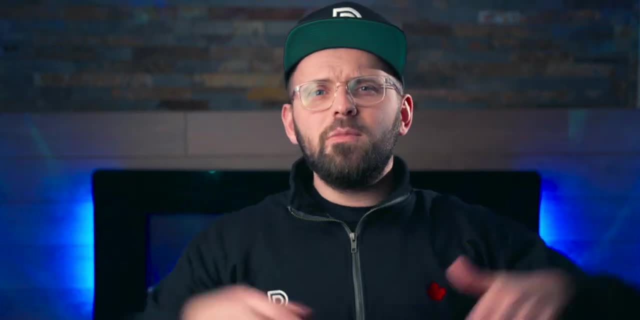 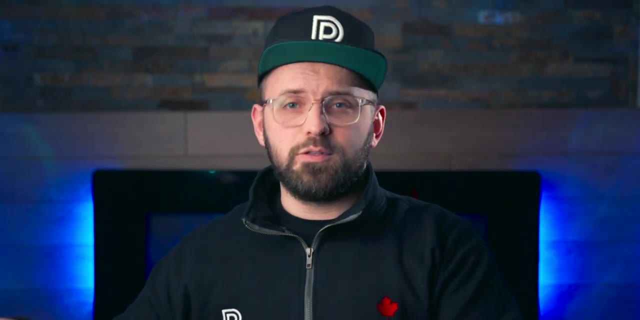 where 0% of the light is reflected off of it. Today's color combos are all by Sherwin-Williams, but no matter what paint company you like to use, you could tint these colors in any product really. So if you're ready to start this dramatic journey with me, 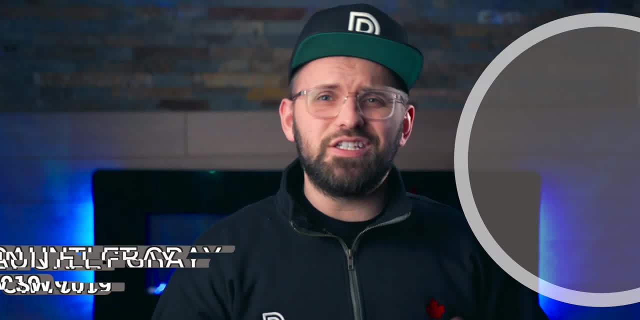 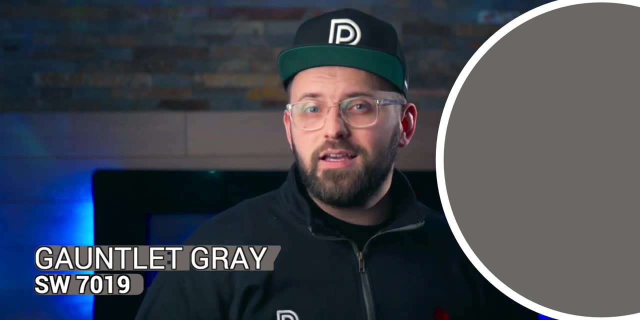 let's get into the first pairing. The first dark color I want to feature is gauntlet gray, SW 1719.. This is one of my favorite dark topes in the Sherwin-Williams catalog. It has an LRV of 17,. 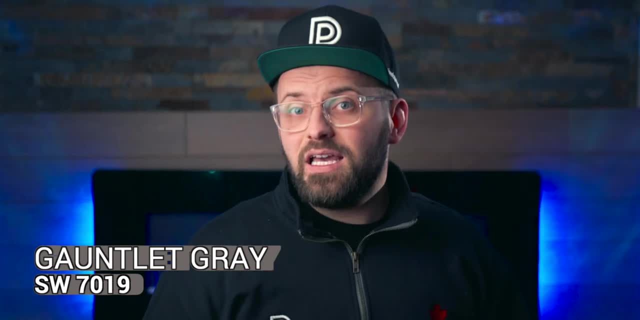 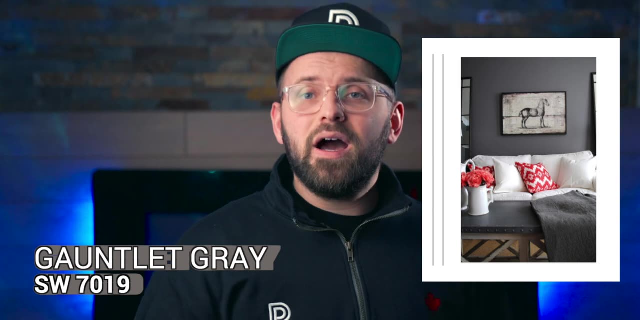 so it's not quite dark enough to seem like an off black, but it's one of your more earthy brown, dark slate grays, which simply translates to a really dark taupe, And it combines a little bit of yellow and a little bit more of red in its undertones. 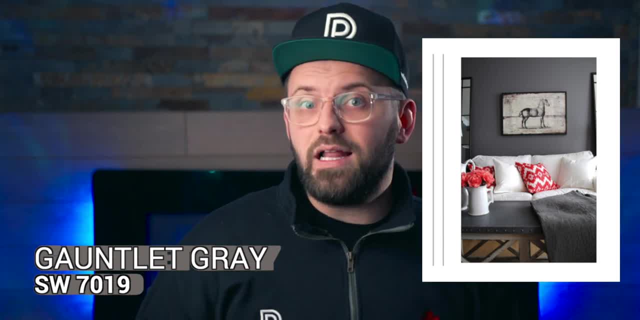 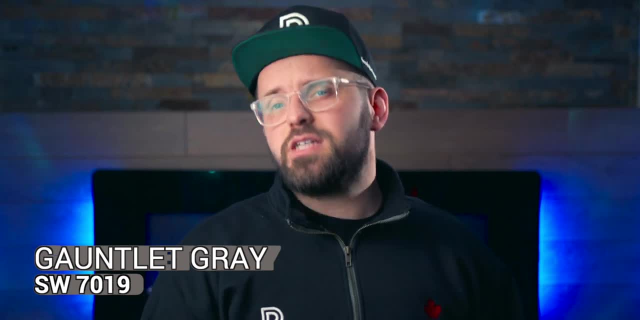 This type of color will always work with the lighter, neutral color palette because, even though it's dark, its undertones categorize it as a neutral based on its makeup. It's one of the more versatile colors you can use at this level of depth. 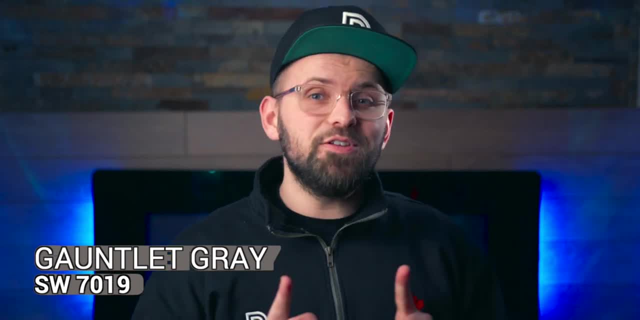 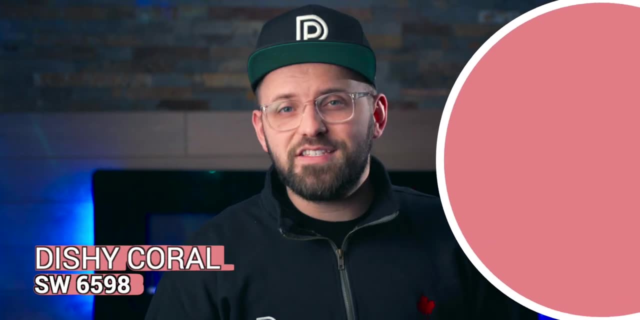 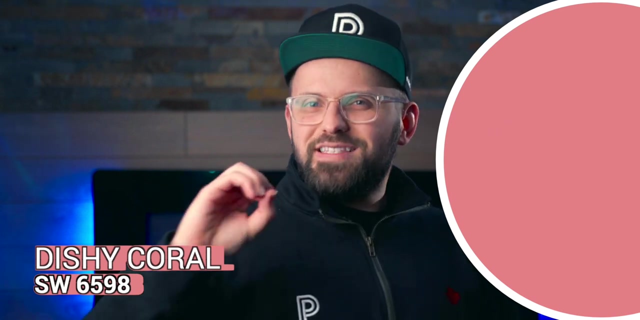 On its own, nothing too groundbreaking here, until we introduce the second part of this color combo, and it's the strawberry milk colored dishy coral, SW 6598.. Coral is such a fun, bright, juicy color to use because it incorporates red with that little dash of orange. 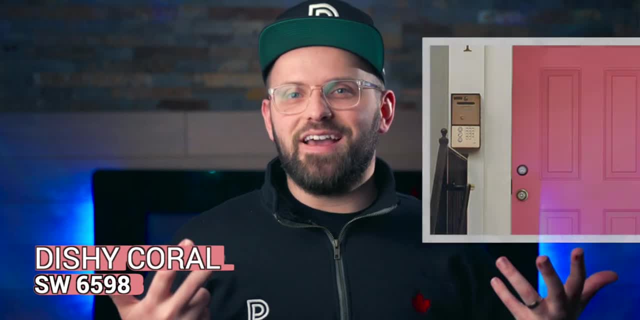 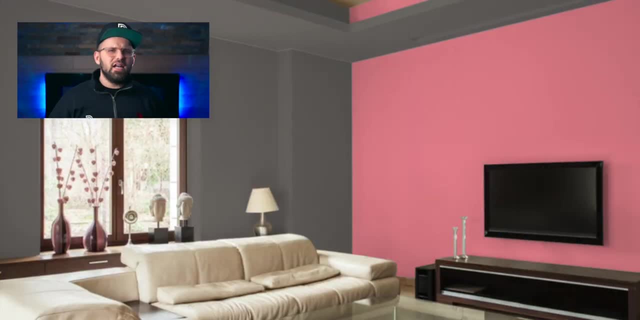 to energize the overall look. It just brings a smile to my face. You can also opt for a more orange dominant coral, but I kind of like the balance in dishy coral and it's because it leans a little more towards the red side. 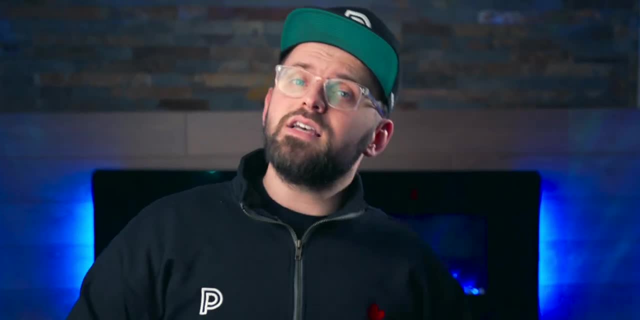 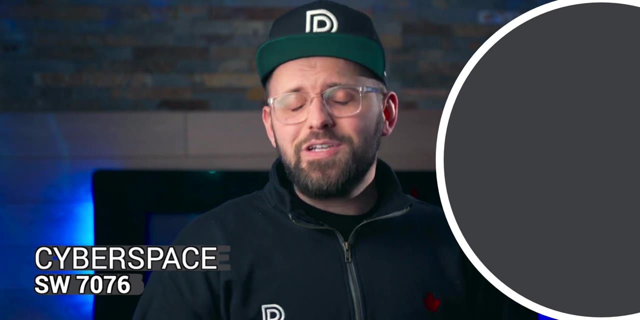 which feels a bit classier to me. The next color pairing utilizes a much darker color in Cyberspace: SW 7076. And with an LRV of six you should get the idea of how dark this color is. It's one of my go-to wrought iron blacks. 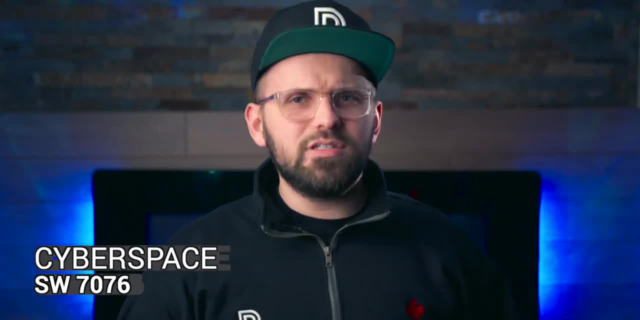 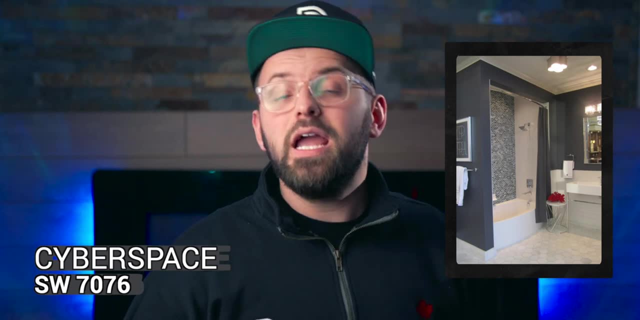 that has a perhaps a subtle blue green tinge to it. maybe, but nothing that would make it feel any less black of a color. It's been featured in many Sherwin-Williams color collections, including the recent 2021 Continuum Color Palette. 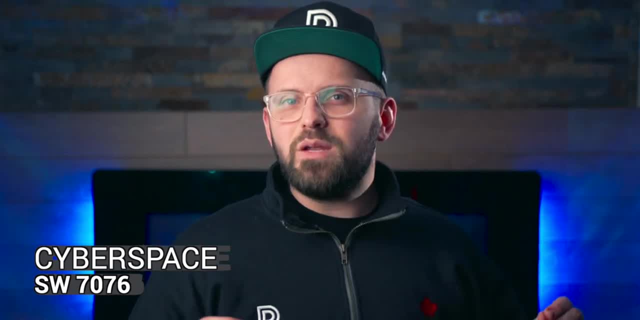 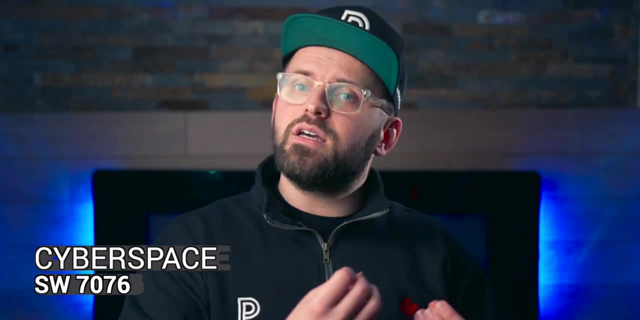 which we spoke about in a previous video. Now, what I like to do when I want to minimize that bit of green that sometimes pops out in Cyberspace is I introduce a paired color that has a bit of green to pull focus a bit. 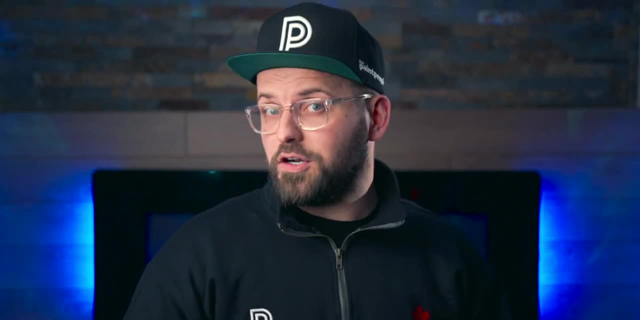 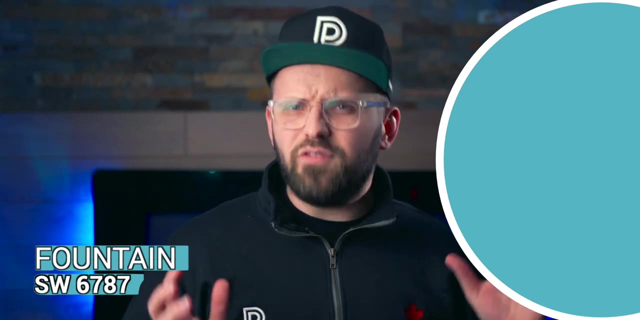 For this combo. I'll accomplish that in the form of a blue color called Fountain SW 6787.. This lovely aquamarine is so fun, so full of life and vibrancy, even though it has a pretty low LRV of 39.. 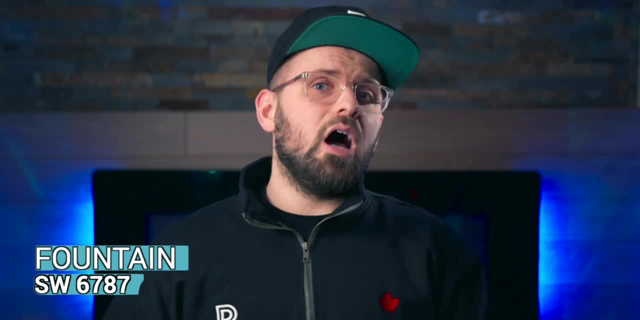 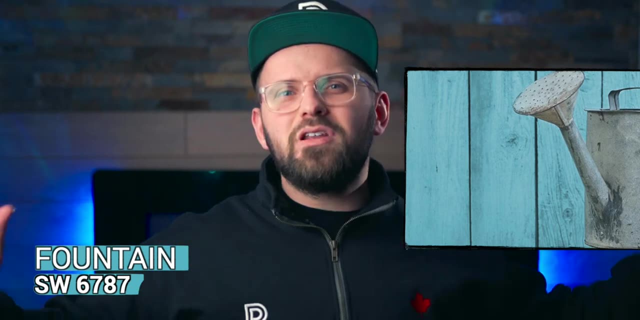 When working with really dark slate grays and blacks, people normally opt to pair them with other grays, or perhaps some taupes or light greys, but why not go with something to cut through the monotony of neutrals? I love the playful nature of this pairing. 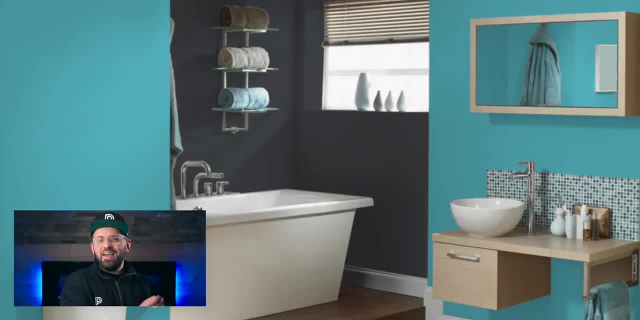 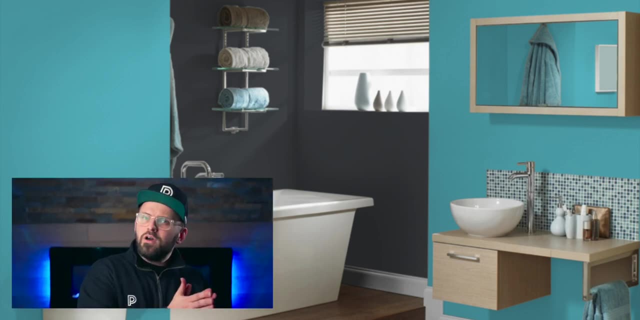 because you have the very serious cyberspace coming together with the super fun fountain. It's not only a fun interpretation of black and blue, but it's the blue that makes Cyberspace look even deeper as a black. The third and final color combo. 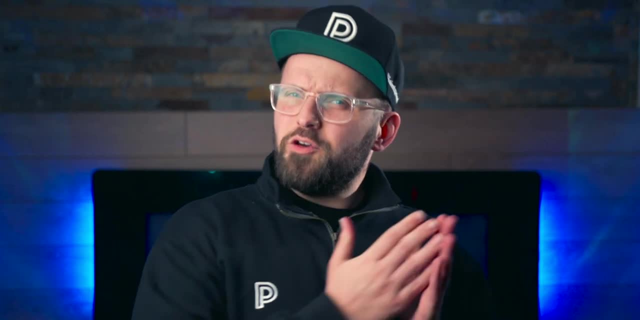 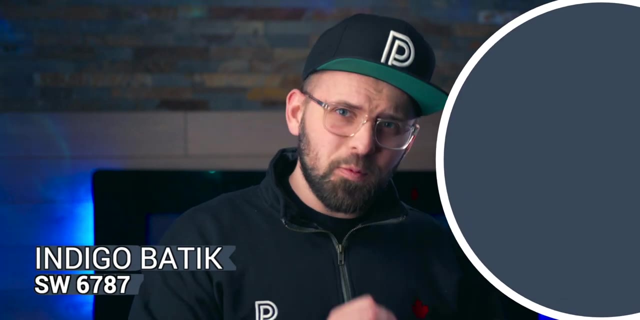 of these dark and daring color choices are sort of a fusion of the previous two With an LRV of eight. the darker color in this grouping is Indigo Batik. This uber dark navy blue is similar to the types of colors you might find. 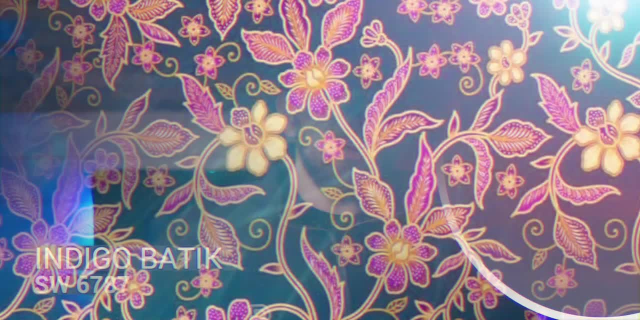 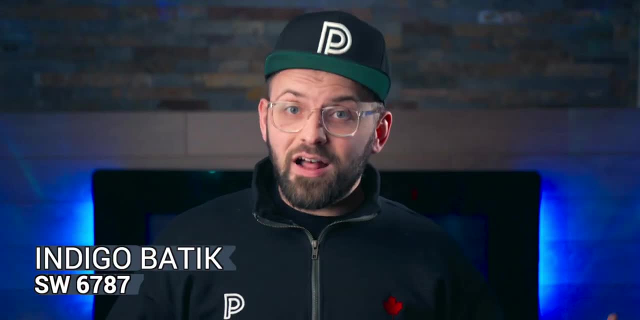 in some beautiful Indonesian batik fabrics. In fact, that's what sort of inspired me to put this combination together, because, after seeing some of these fabrics during my brief stay in Bali, I was floored by how striking some of these color combinations were. 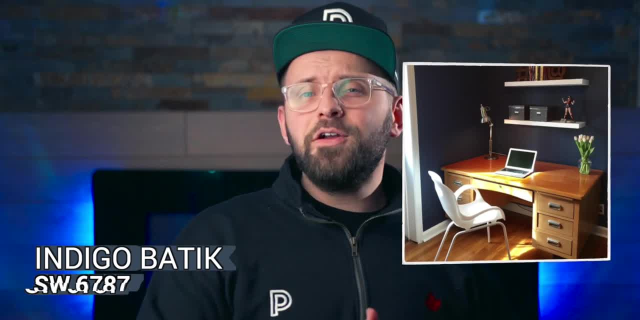 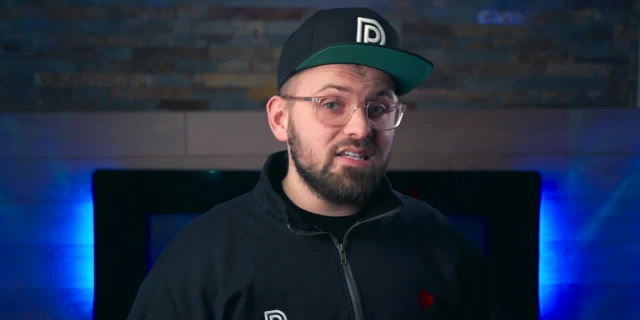 And I absolutely loved the history behind them. For our lighter color in this pairing we're going all the way up to a 50 LRV, which is technically the lightest color in this video, but that doesn't mean it's boring. 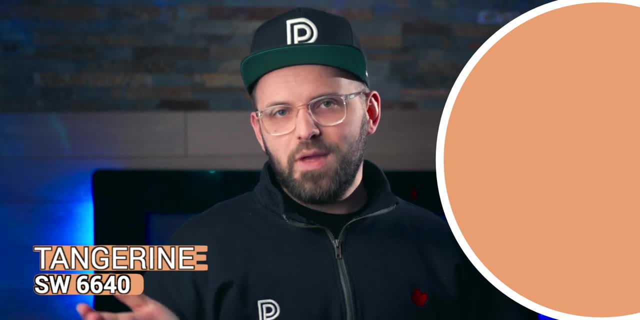 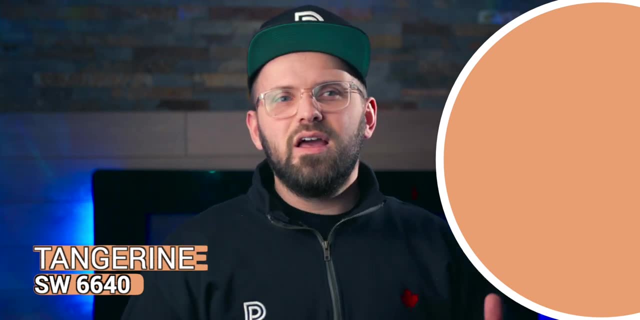 Tangerine SW6640.. So we touched on coral earlier on. This color goes all the way to orange, but there still seems to be that subtle touch of pinky, peachy pinkiness as well, And that prevents it from feeling. 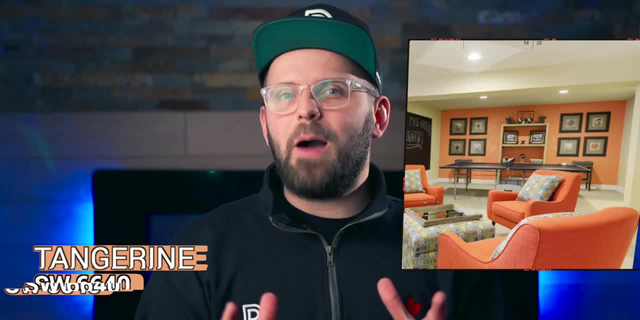 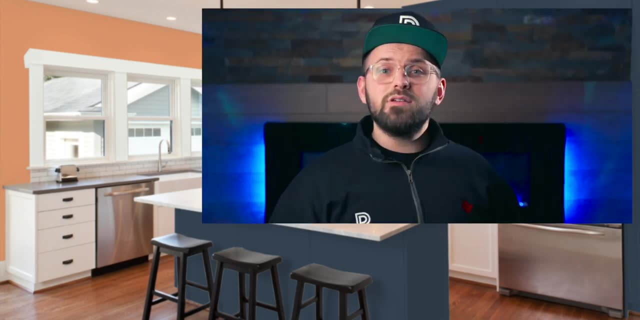 too fluorescent and overbearing. The two together are so complimentary, so engaging, that they really do a fantastic job at livening up any space you use them in. There's some more color combos coming at you right over here, And these ones are also pretty fun.